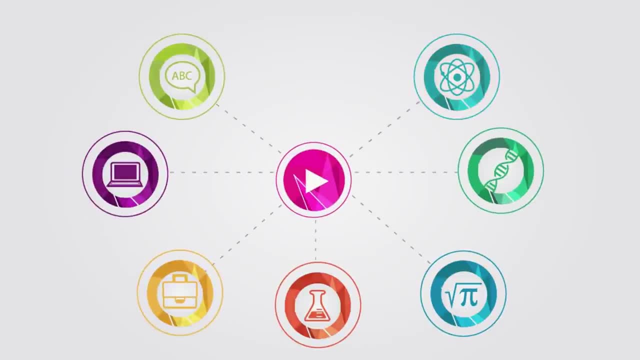 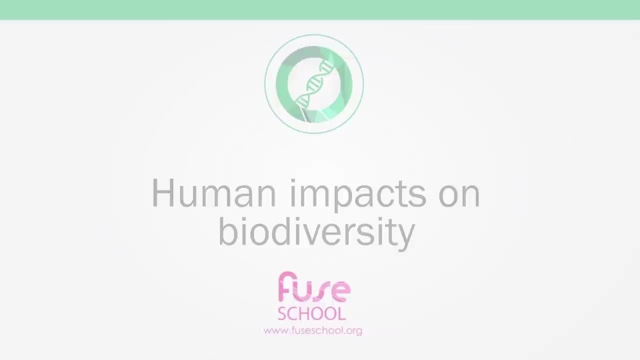 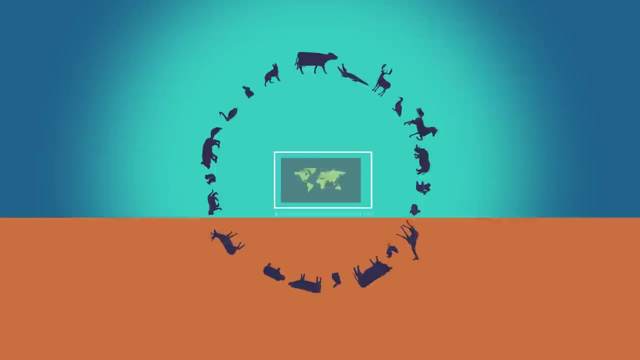 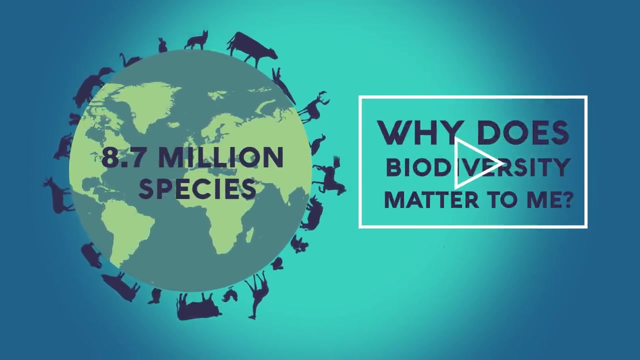 Biodiversity is the variety of life, as we saw in this video. There are thought to be 8.7 million species on planet Earth and, as we saw in this video, biodiversity is of utmost importance to humans. The loss of one key species can have a detrimental impact on many. 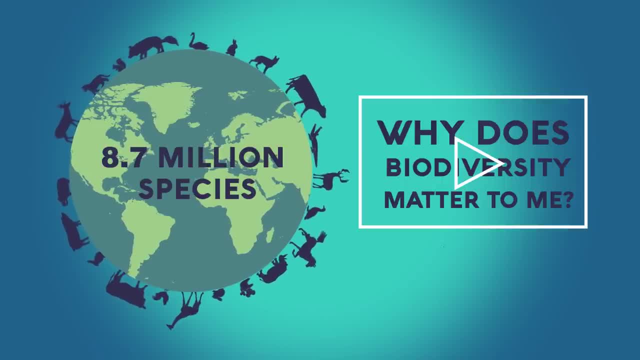 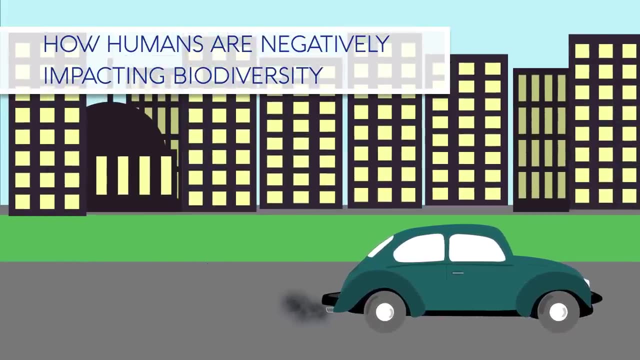 levels, from other species of animals to plants, to the physical environment. as shown by wolves, Human activities are reducing biodiversity. Our future depends upon maintaining a good level of biodiversity, and so we need to start taking measures to try and stop the reduction. 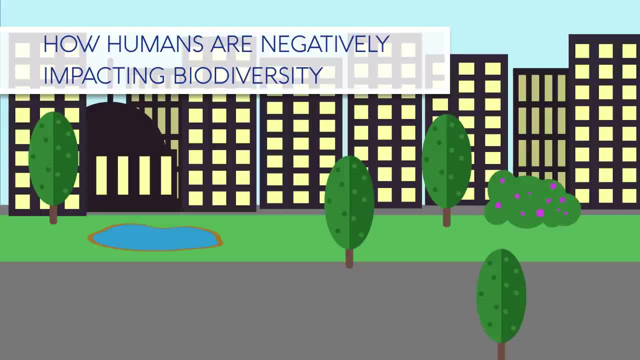 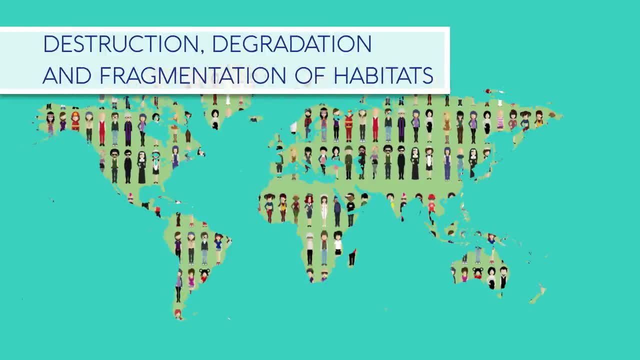 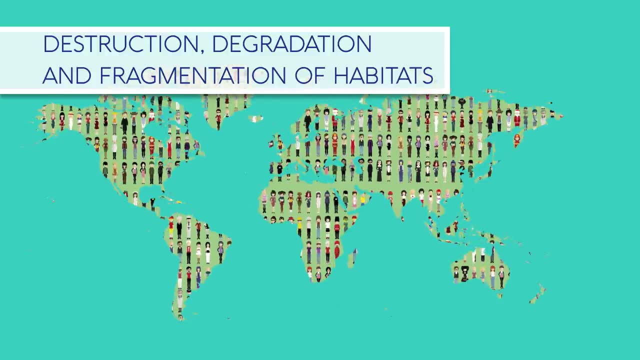 In this video we're going to look at how humans are negatively impacting biodiversity. Here are some of the main human-induced threats facing biodiversity. As the world population has grown from 1.5 billion to 1.5 billion in 1900, to nearly 7.5 billion people today, unsurprisingly, the land use has changed. 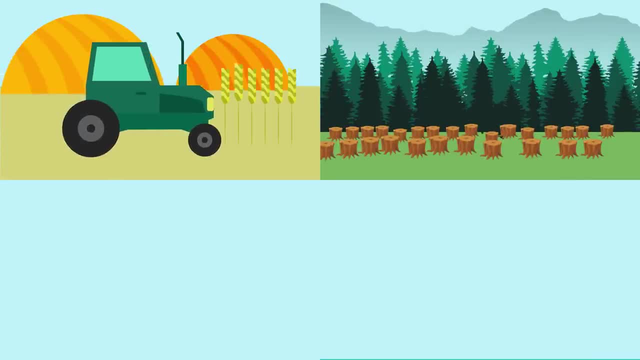 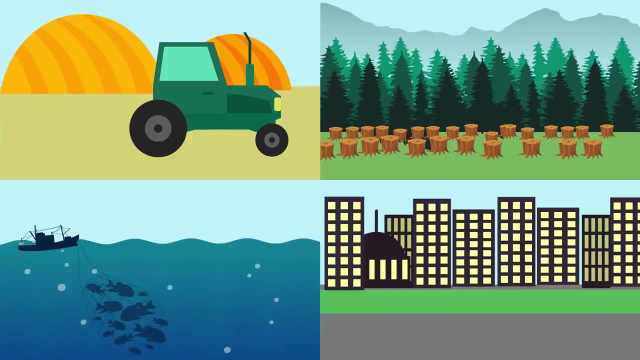 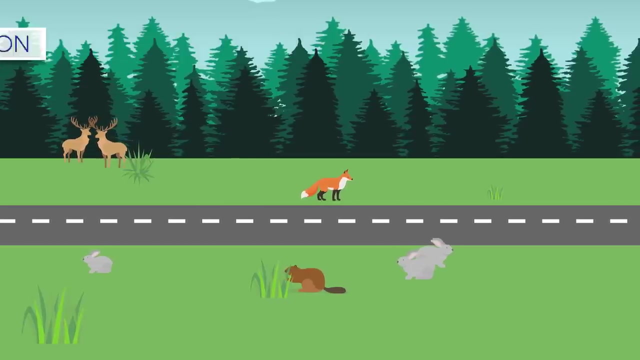 Habitats have been destroyed in favor of agriculture, forestry, fishing, urbanization and manufacturing. Unsurprisingly, habitat loss has greatly reduced species richness. Habitat fragmentation has also meant that populations have been split into smaller subunits, which then, when faced by challenging circumstances, have not been able to adapt and 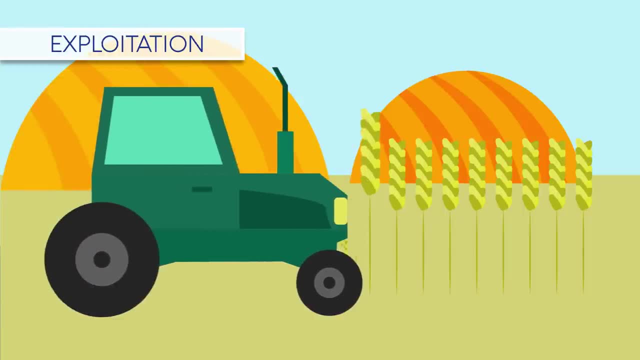 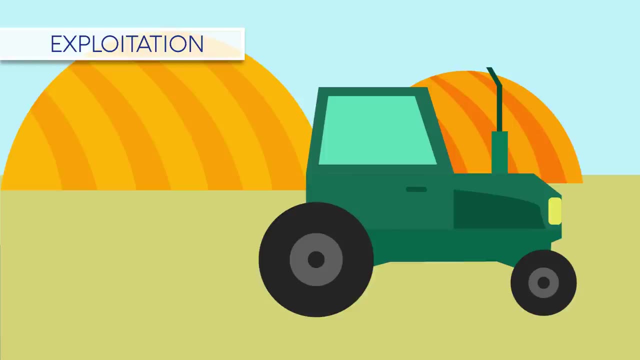 survive After habitat loss. over-harvesting has had a huge effect on biodiversity. Humans historically exploit plant and animal species for short-term profit. If a resource is profitable, we develop more efficient methods of harvesting it, inevitably depleting the resource, As is currently happening with fishing and logging. 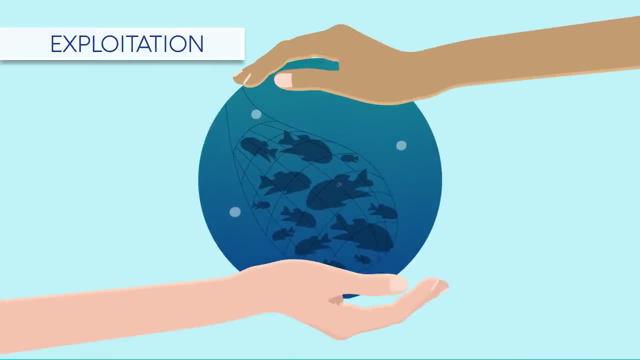 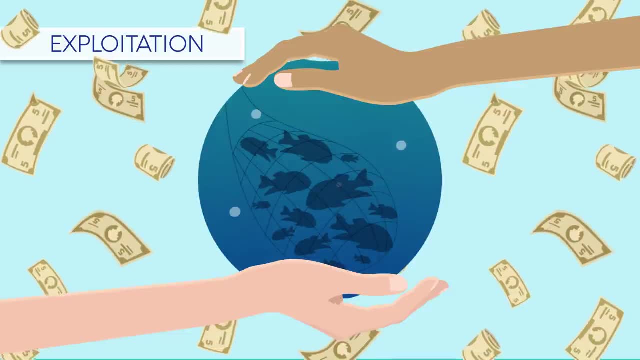 The demand is then outstripped by the supply, and so the resources are destroyed. The demand is then outstripped by the supply, and so the resources are destroyed. This increases the incentive to extract the resource and leads to the final collapse of the population. 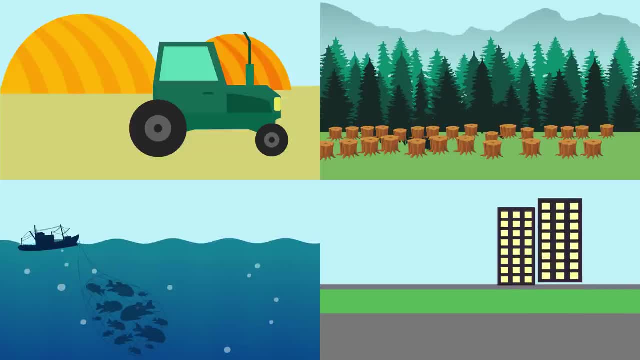 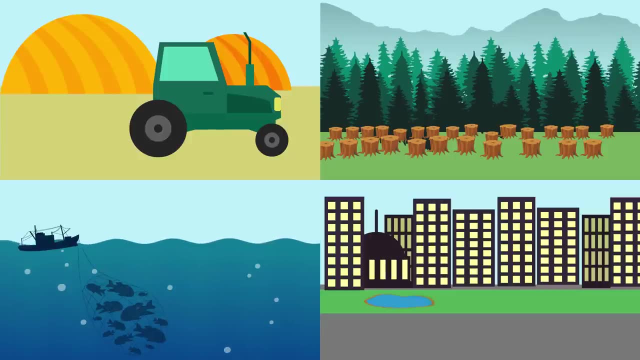 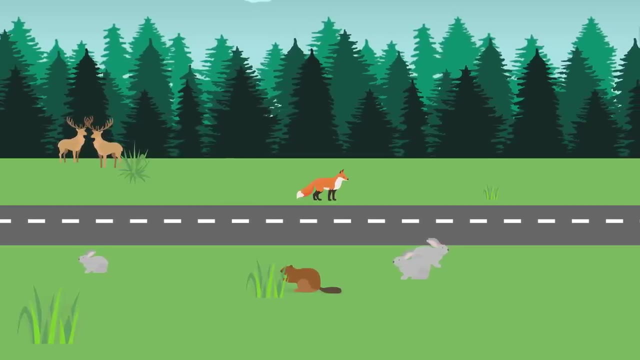 agriculture, forestry, fishing, urbanisation and manufacturing. Unsurprisingly, habitat loss has greatly reduced species richness. Habitat fragmentation has also meant that populations have been split into smaller sub-units which then, when faced by challenging circumstances, have not been able to adapt and survive. 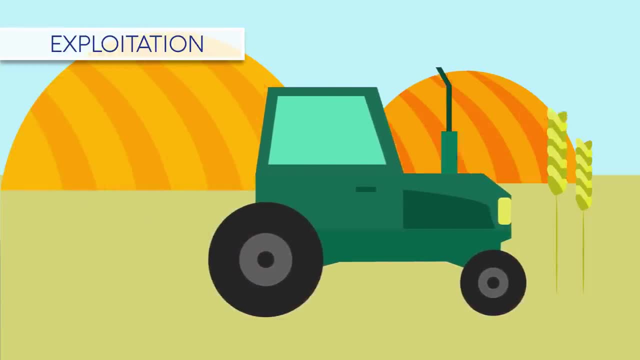 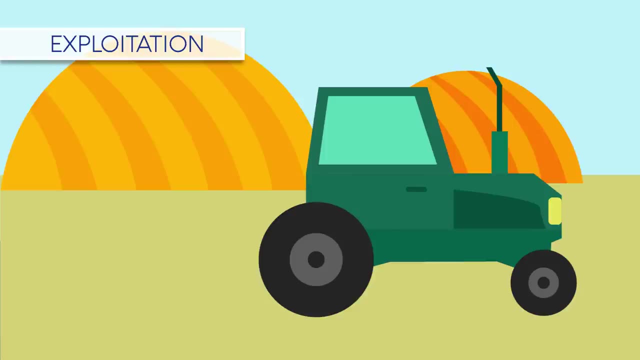 After habitat loss, over-harvesting has had a huge effect on biodiversity. Humans historically exploit plant and animal species for short-term profit. If a resource is profitable, we develop more efficient methods of harvesting it, inevitably depleting the resource, As is currently happening. 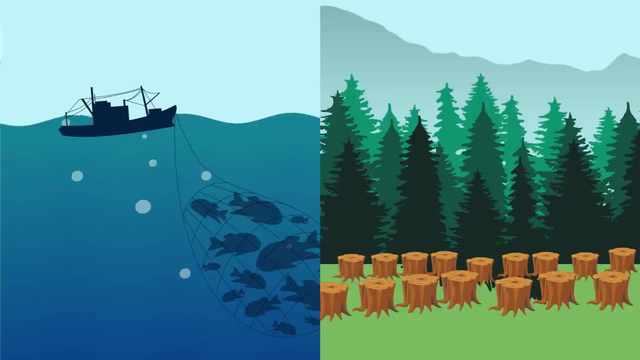 with fishing and logging. the exploited species then needs protection. The difficulty is that the demand then outweighs the demand. In this video, we are going to look at some of the main human-induced threats facing biodiversity, As the world population has grown from 1.5 billion to nearly 7.5 billion people today, unsurprisingly. 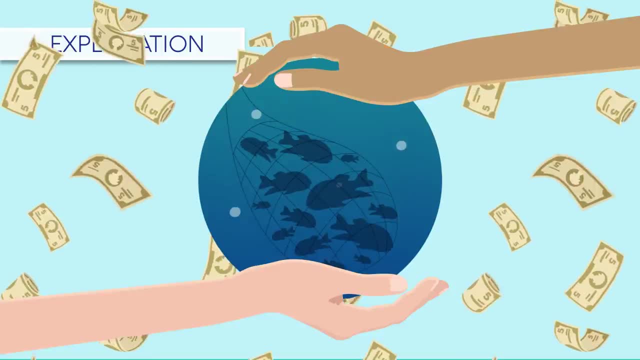 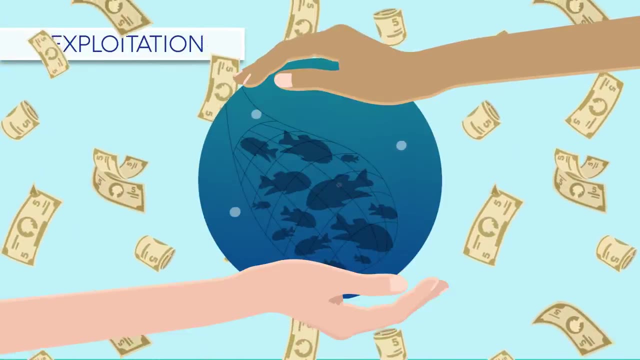 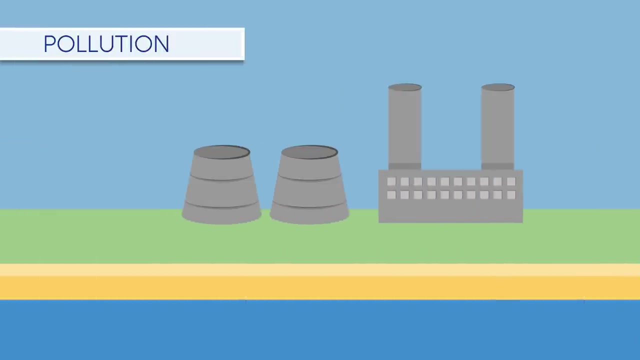 the demand then outstrips the supply, And so the resource value rises. This increases the incentive to extract the resource and leads to the final collapse of the population, As happened with whales, elephants, spotted cats, cod, tuner and many more species. 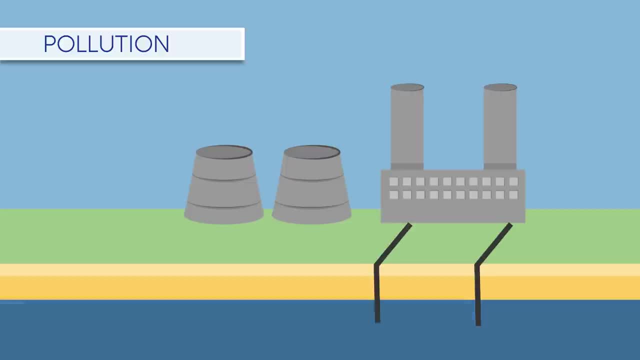 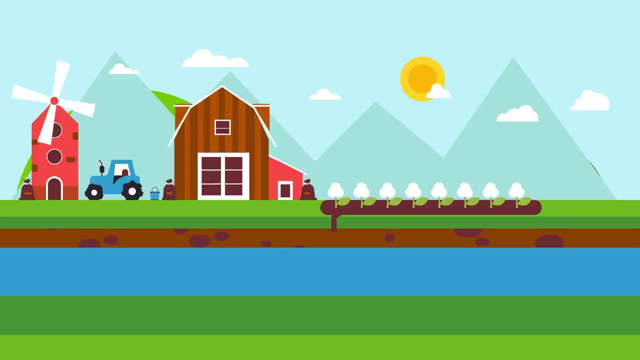 Human activities are polluting the air and water. Toxics discharged into water from industrial processes unsurprisingly has a negative effect on local aquatic species by killing, destroying, weakening or affecting their ability to reproduce. another big water pollution problem is eutrophication, which we look at in detail in this video. phosphorus and nitrogen in fertilizers. 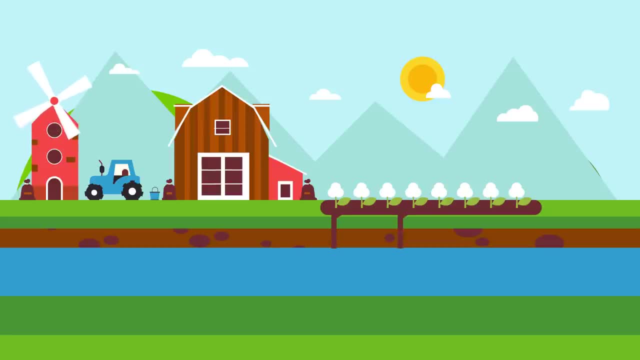 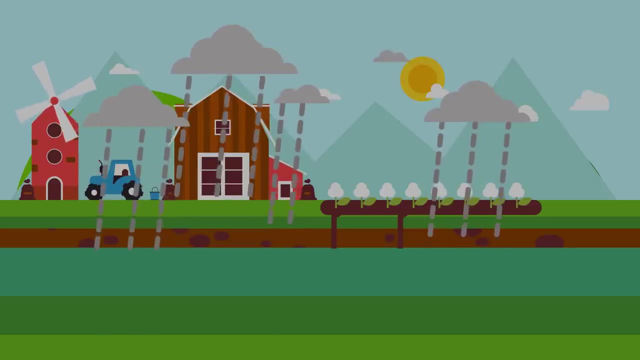 run off agricultural fields and pass into rivers. these surplus nutrients cause algae to bloom, which then starves other aquatic species of oxygen and light, causing them to die. acid rain is the consequence of humans polluting the air. this causes lakes and water bodies to become more acidic, killing fish, mollusks, amphibians and many other species. a huge impact humans have had on 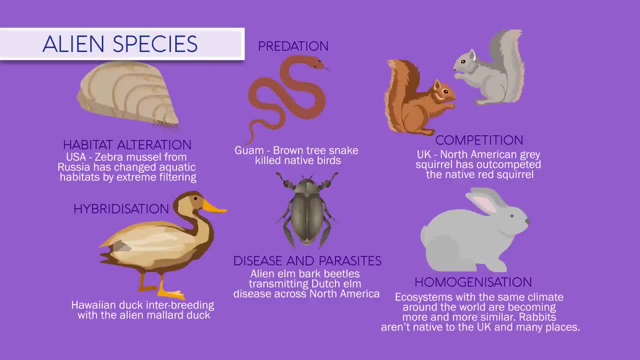 planet earth is introduction of alien species to habitats. in fact, it is estimated that on any given day, there are 3 000 species in transit aboard ocean-going vessels. alien species can cause problems in a number of ways. pause the video and have a look. throughout the earth's history, there have been periods.